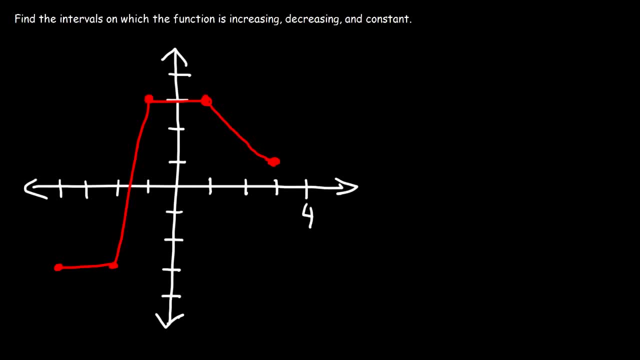 In this video we're going to focus on increasing and decreasing functions. So a function is increasing when the graph is going up as you move from left to right. It's constant when it's just maintaining the same y-value if it's horizontal, and it's decreasing if it's going down as you move from left to right. So in this 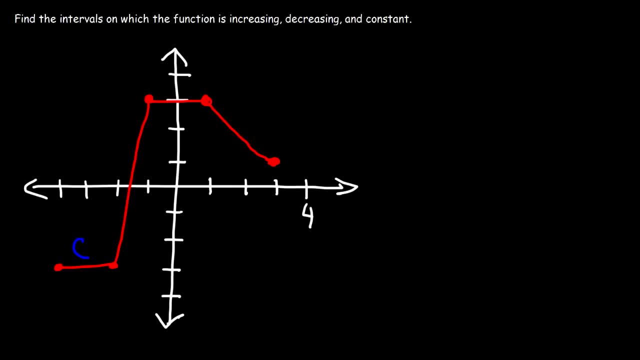 region the function is relatively constant. I know my graph is not perfect, but we're going to be reasonable with it. In the second part it's increasing, it's going up, In the third part it's constant and then in the last part it's decreasing. 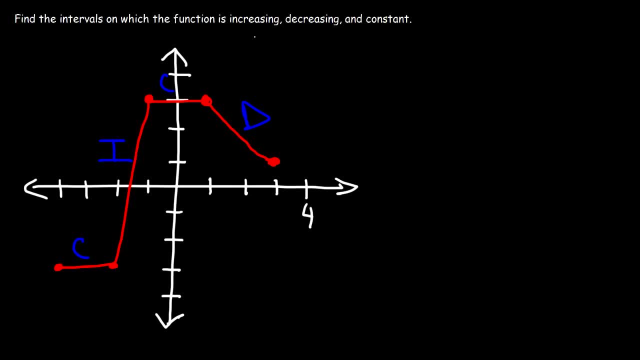 it's going down, So let's focus on the intervals where it's increasing first. So it's increasing, and we're going to use the X values to describe it. It's increasing starting from negative two and ending negative 1, so we're going to write negative 2 to negative 1. now what? 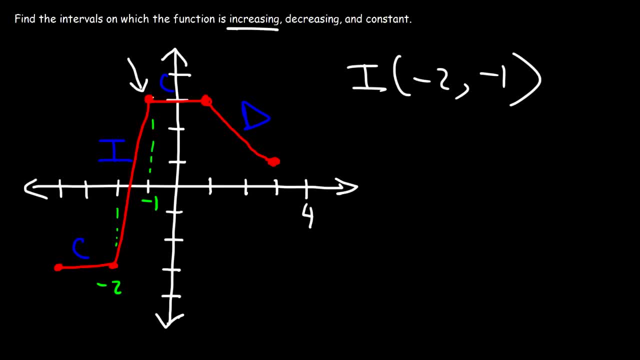 doesn't include negative 2 or negative 1, because at this exact point you can't say it's increasing our constant. so we're going to use parentheses. now let's talk about when it's decreasing. so it's decreasing when it's going down and it's 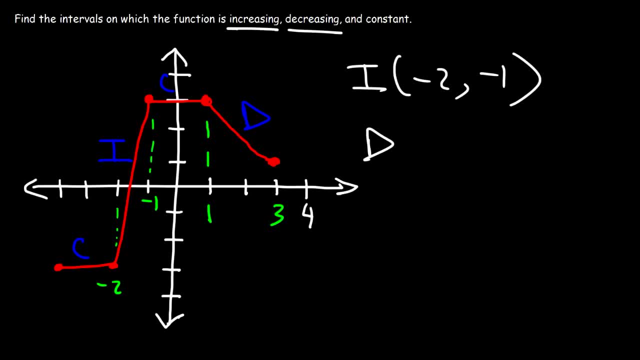 going down, starting that one but ending that three, so it's decreasing from one to three. now, when is the function constant? let me use a different color to describe it. so it's constant, starting from negative 4 to negative 2 and starting back up from negative 1 to 1. so for the first part it's constant from. 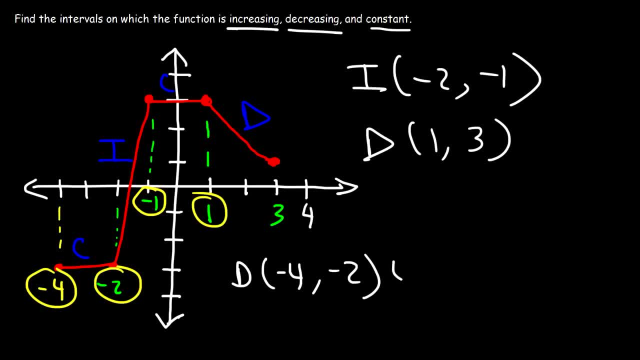 negative 4 to negative 2, and then union. we need to connect that with the second part, where it's constant, and that's from negative 1 to 1, you and so that's it. so now you know how to determine when the function is decreasing, when it's increasing and when it's constant. you know what I put D for. 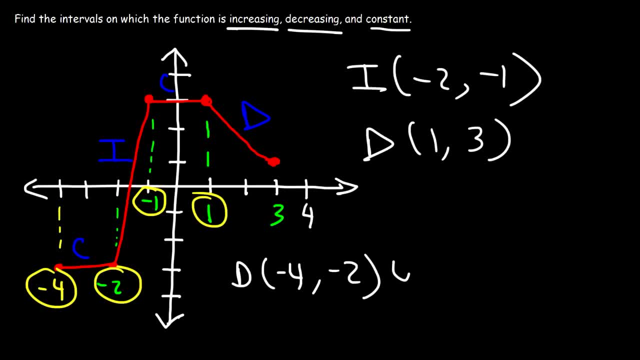 negative 4 to negative 2, and then union. we need to connect that with the second part, where it's constant, and that's from negative 1 to 1, you and so that's it. so now you know how to determine when the function is decreasing, when it's increasing and when it's constant. you know what I put D for. 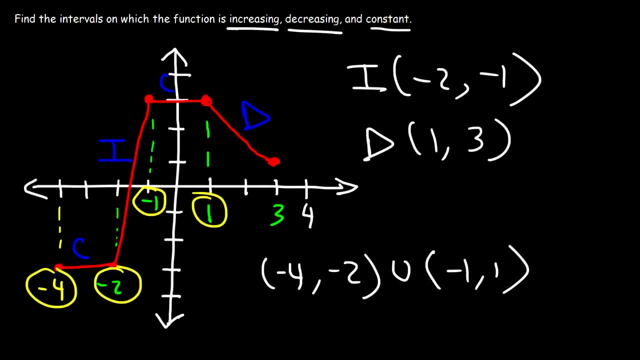 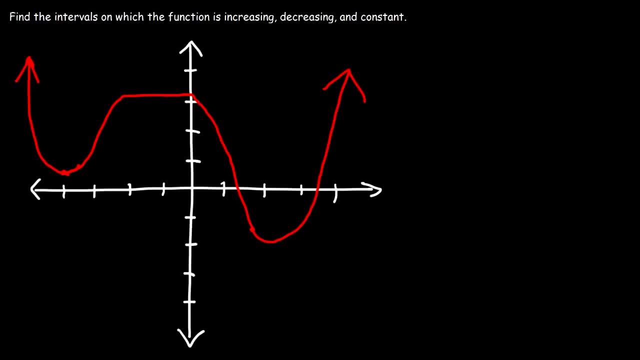 this one. this should be C for constant, so let's just fix that. so let's work on some more examples. let's try this one. so notice that in the first part the function is increasing, and when it's increasing it's constant. so that's it so. 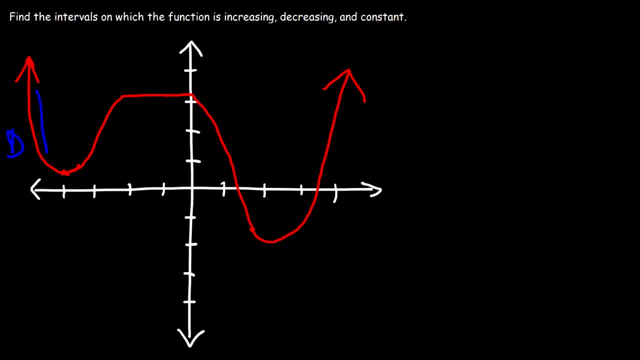 the function is decreasing at this section and then in this section it's an increase in either four increases and then it's constant, and then after that it's decreasing. let's put a D there. and then it goes up. it's increasing. so let's determine the intervals with. the function is increasing first, so it's. 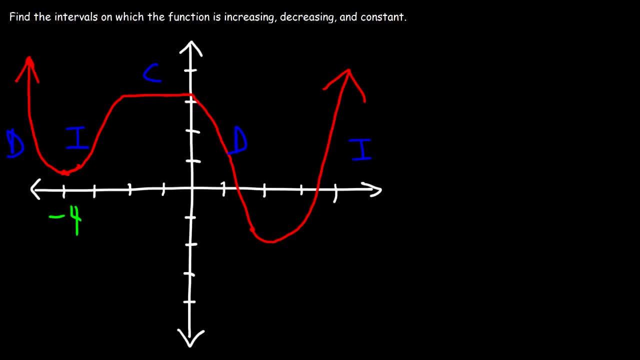 increasing, starting around 3 and someday Douglas starting, and we go from on select around negative 4- doesn't have to be exact- and then it stops approximately at negative 2 and then it increases again, starting around 2 ish, and we have an arrow. so that's going to continue on to infinity. so we could say that it's. 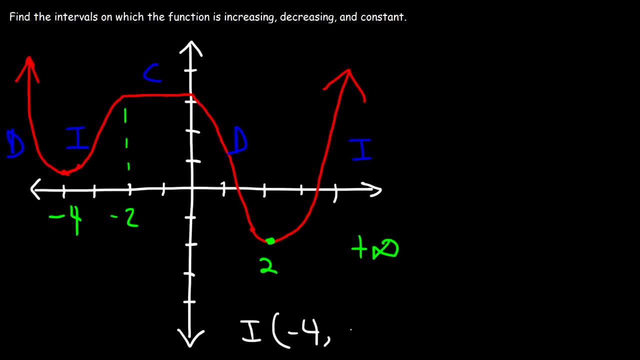 increasing, starting from negative 4 to negative 2. that's the first part, and then union. let's connect it to the second part, from 2 to infinity. now, when is the function decreasing? so it's decreasing in this section all the way to the left. it starts from negative infinity and then it stops decreasing at. 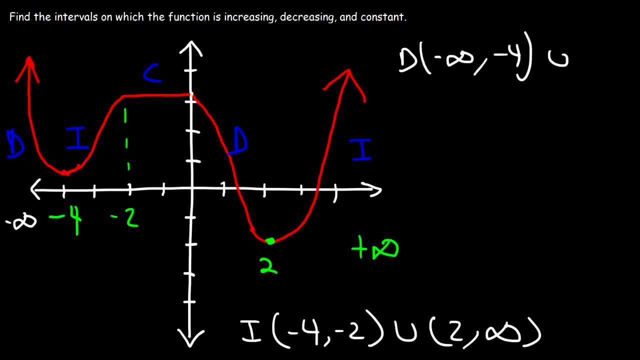 negative 4, and then it starts back up around 0. that's an X value of 0 to 2. let me write that better now. it's constant only from negative 2 to 0, and that's it. so here's the last example finding. 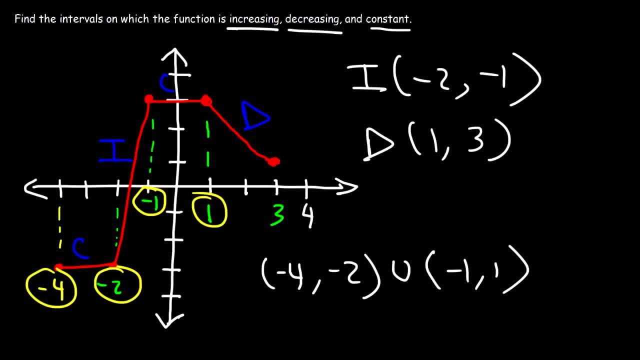 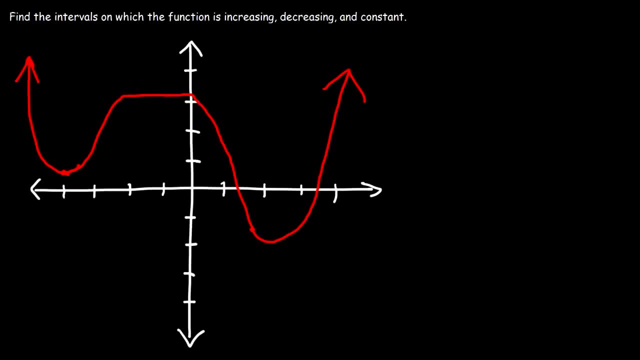 this one. this should be C for constant. so let's just fix that. so let's work on some more examples. let's try this one. so notice that in the first part the function is decreasing and when it's increasing it's constant. so that's it is decreasing at this section and then in this section it's increasing. so I'm 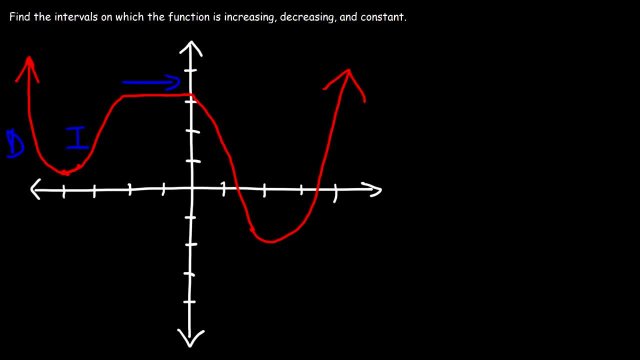 going to put either for increasing, and then it's constants and then after that it's decreasing. so let's put a D there, and then it goes up. it's increasing, so let's determine the intervals where the function is increasing first. so it's increasing starting around the next step, and then it's increasing, it's increasing. 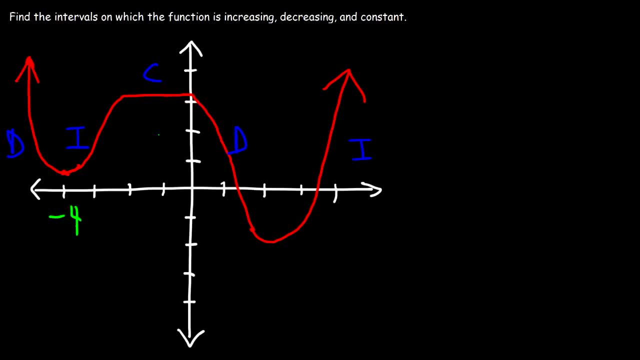 around negative 4- doesn't have to be exact- and then it stops approximately at negative 2 and then it increases again, starting around 2 ish, and we have an arrow, so that's going to continue on to infinity. so we could say that it's. 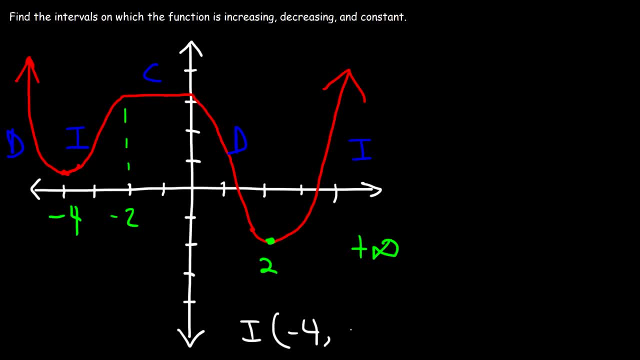 increasing, starting from negative 4 to negative 2. that's the first part, and then union. let's connect it to the second part, from 2 to infinity. now, when is the function decreasing? so it's decreasing in this section all the way to the left. it starts from negative infinity and then it stops decreasing at. 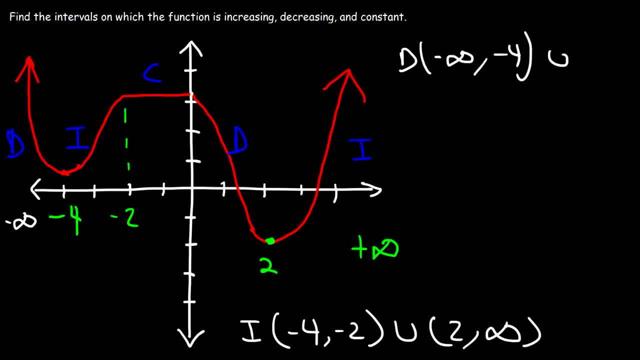 negative 4, and then it starts back up around 0. that's an X value of 0 to 2. let me write that better now. it's constant only from negative 2 to 0, and that's it. so here's the last example. find the intervals on which the function is.